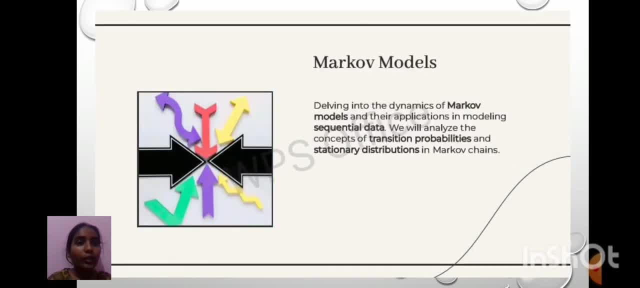 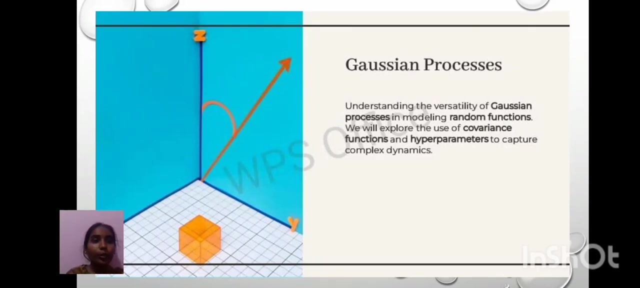 Macro models: Delving into the dynamics of macro models and their applications in modeling sequential data. we will analyze the concepts of transition probabilities and stationary distributions in macro chains. macrochains- Gaussian processes- Understanding the versatility of Gaussian processes. in modeling random functions, we will explore the use of covariance functions and hyperparameters. 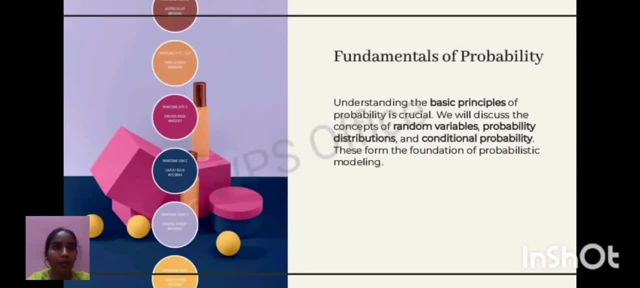 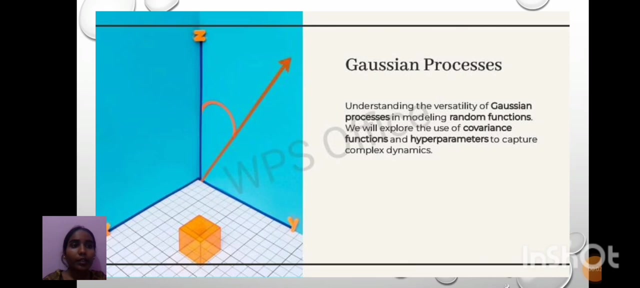 to capture complex dynamics. Fundamentals of probability: Understanding the basic principles of probability is crucial. We will discuss the concepts of random variables, probability distributions and conditional probability. These form the foundation of probabilistic modeling. Gaussian processes: Understanding the versatility of Gaussian processes in modeling. 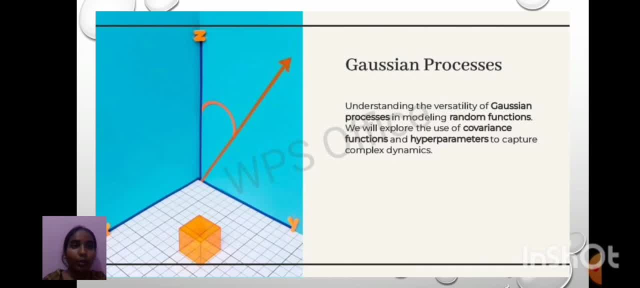 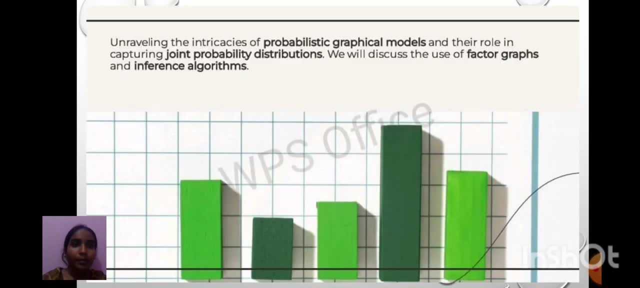 random functions. we will explore the use of covariance functions and hyperparameters to capture complex dynamics, Unraveling the intricacies of probabilistic graphical models and their role in capturing joint probability distributions. we will discuss the use of factor graphs and inference algorithms. 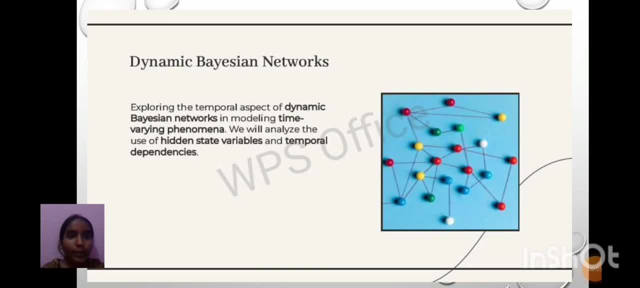 Dynamic Bayesian networks: Exploring the temporal aspect of dynamic Bayesian networks in modeling time-varying phenomena. we will analyze the use of hidden state variables, Unraveling the intricacies of probabilistic graphical models and their role in capturing joint probability distributions. we will explore the concepts of variance variables and temporal 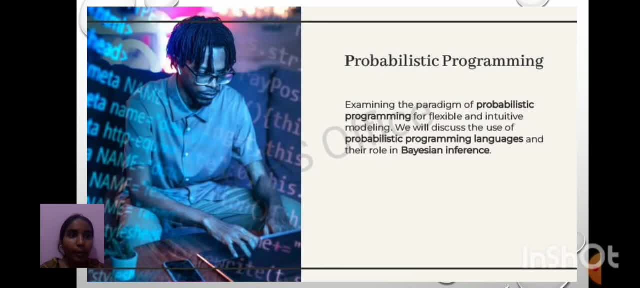 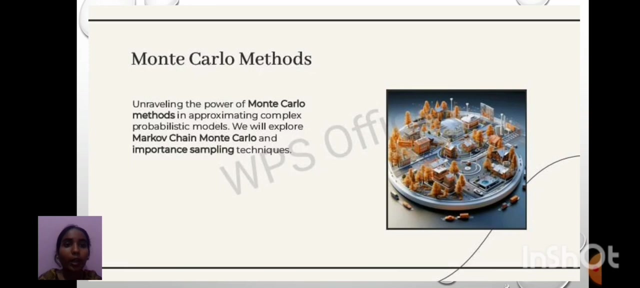 dependencies. Probabilistic programming: Examining the paradigm of probabilistic programming for flexible and intuitive modeling. we will discuss the use of probabilistic programming languages and their role in Bayesian inferences. Monte Carlo methods: Unraveling the power of Monte Carlo methods in approximating complex probabilistic models. we will explore the 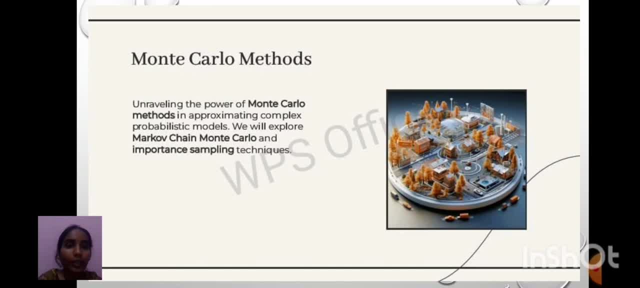 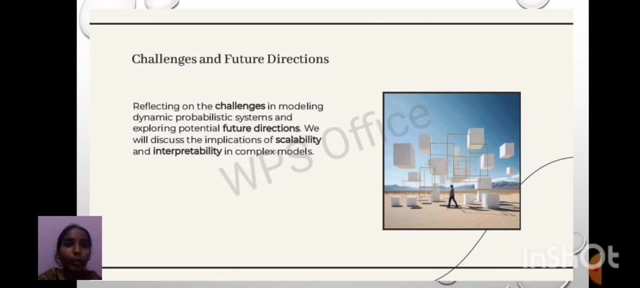 ahhping途 networks. Thank you for watching this video. Challenges and Future directions: Reflecting on the challenges in modeling dynamic probabilistic systems and exploring potential future directions. We will discuss the implications of scalability and interpretability in complex modelsducation and code change.